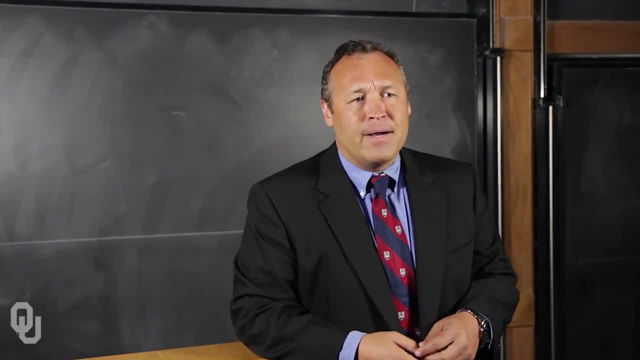 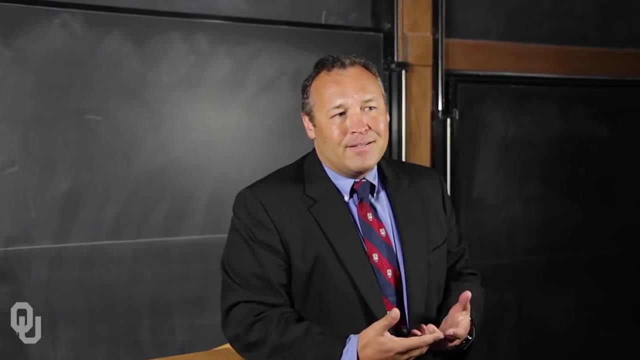 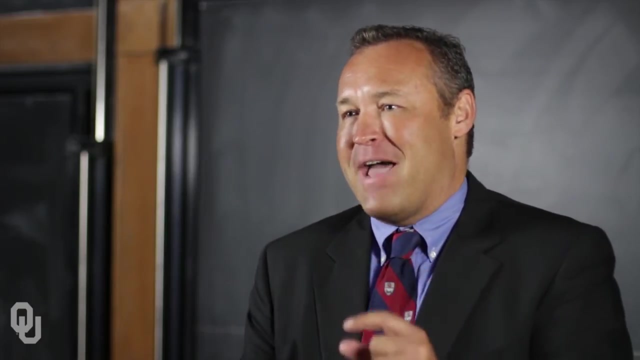 Chemists study chemical compounds and reactions among those compounds. Physicists study things like force and energy. Astronomers study the stars. Social scientists study people, which I think makes our job harder. The helium atom hasn't changed in a thousand years. It still looks the same. 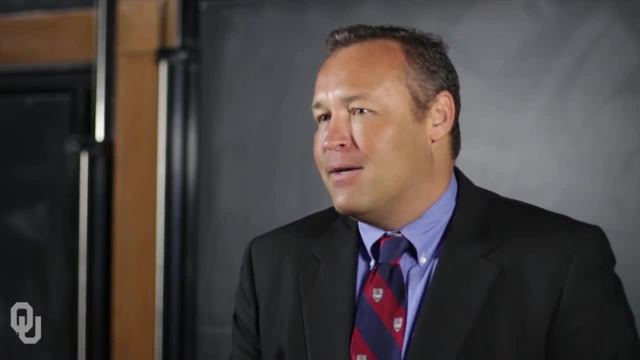 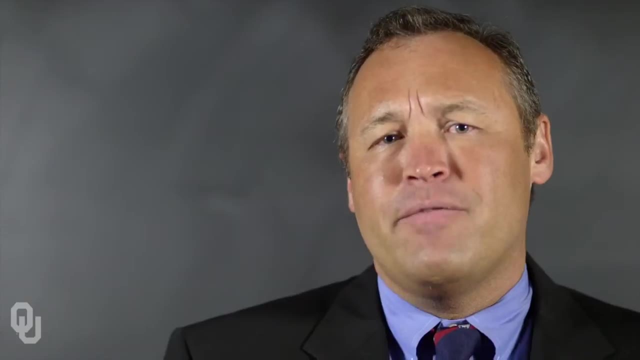 People change all the time. They're really hard to study, So our job is pretty tough. In this class, we're going to talk about how to study human behavior and the techniques that we've learned over the years to study human behavior. 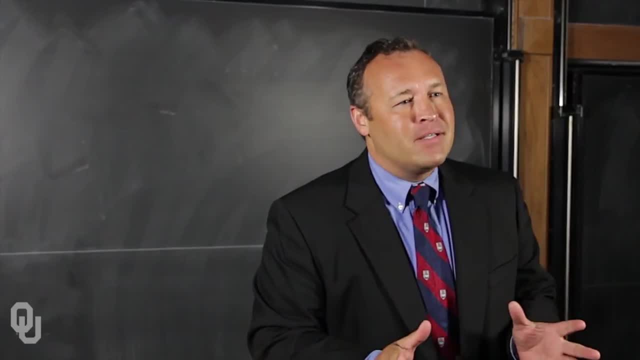 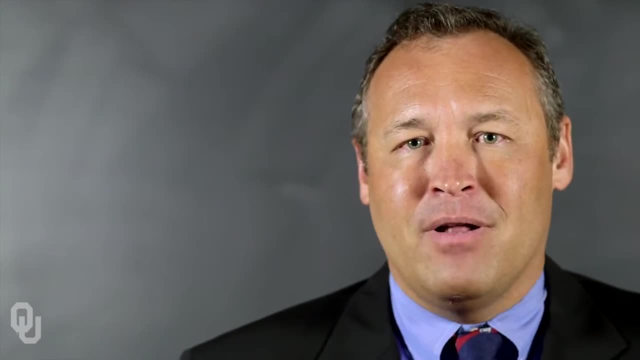 One of the things I discovered when I was learning statistics is that I've been using statistics my whole life. When I was watching hockey as a young person, I knew how to calculate things like goals against average. When I watched baseball, I knew how to calculate certain statistics there. 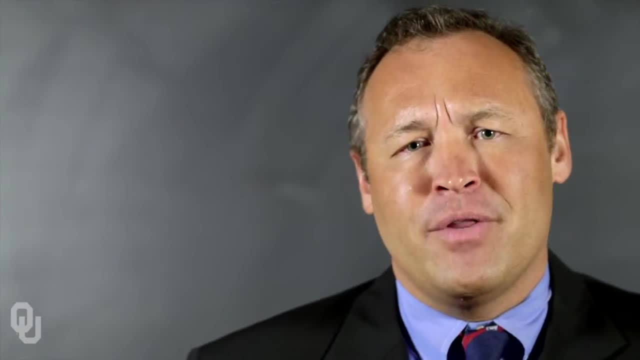 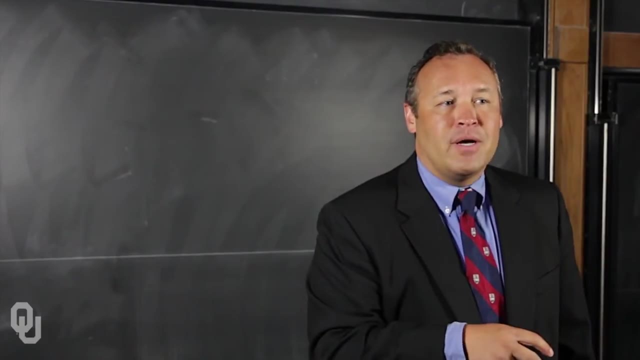 If you're any kind of sports fan, if you read the news, you'll know that statistics are everywhere In this class you're going to have a lot of fun learning about how statistics work in the study of sociology, But you're also going to see how statistics are all around you, how everyone's using them, how you're using them. 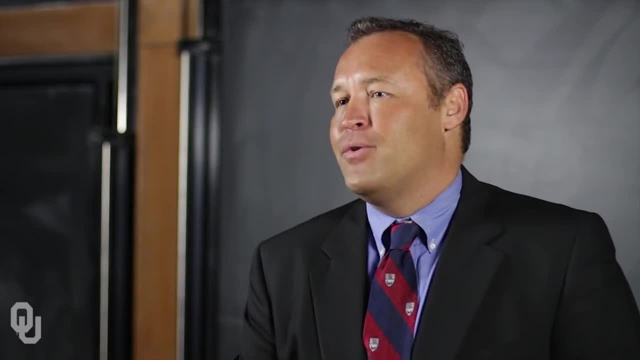 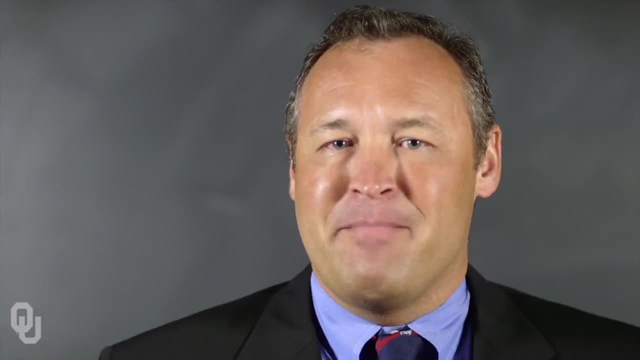 You're going to learn how to calculate those statistics and how they're used in the study of social science. If you're anything like me when I was an undergraduate, the thing that's going to scare you about statistics is the math part. I'm going to confess I'm not a very good math person right now. 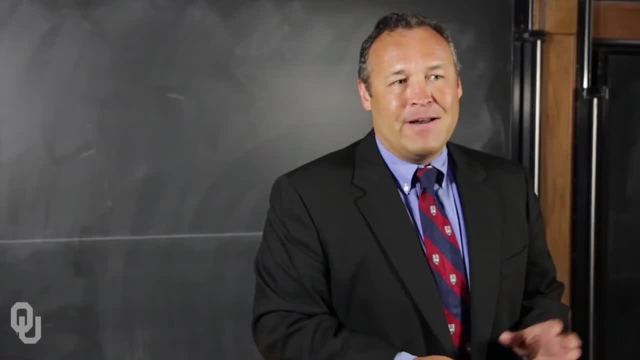 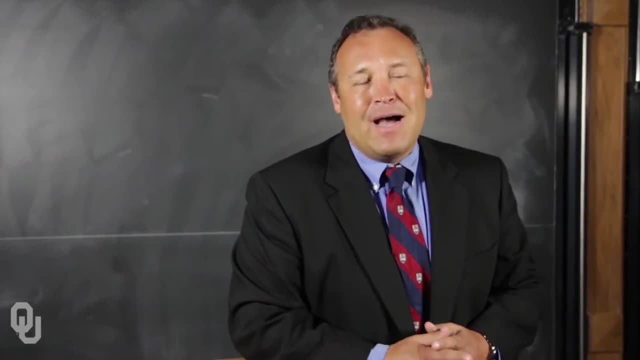 And when I was an undergraduate, I was really afraid of math. In fact, never took any math classes. in college, I never took any math classes until I got to graduate school and took statistics classes. I can guarantee you, though, you're going to survive this class. 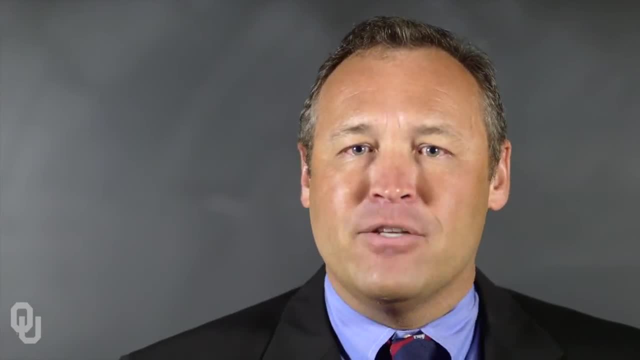 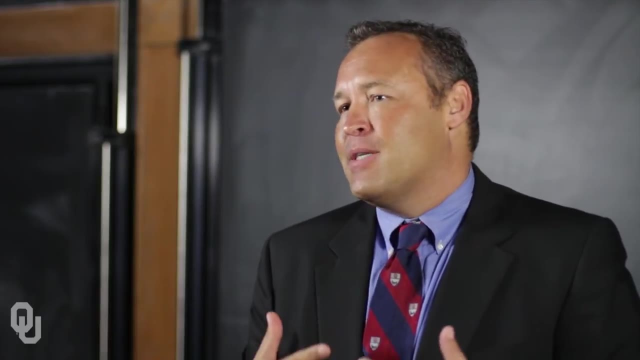 If you can add, subtract, multiply, divide, take the square root of something or square something you're going to do just fine, All right. well, who's teaching this class? Well, I'm going to be doing some introductory videos for most of the lesson units, And my goal here is to give you a broad 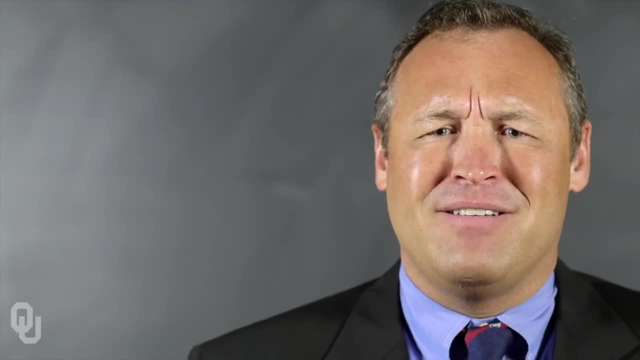 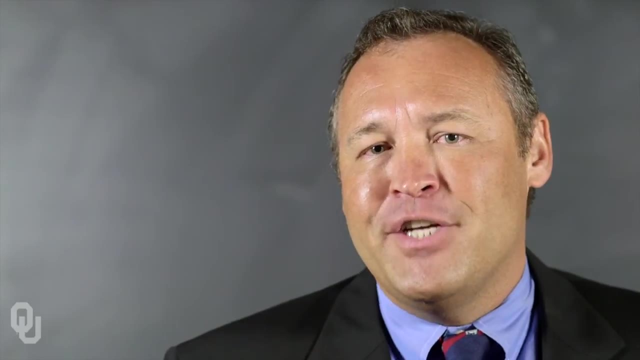 overview of what we're learning about in that unit. I'm not going to teach you how to calculate statistics. I'm going to tell you how those statistics are used, what they mean. My colleague, Mitch Peck, is actually going to teach you about the statistics themselves. He will actually be 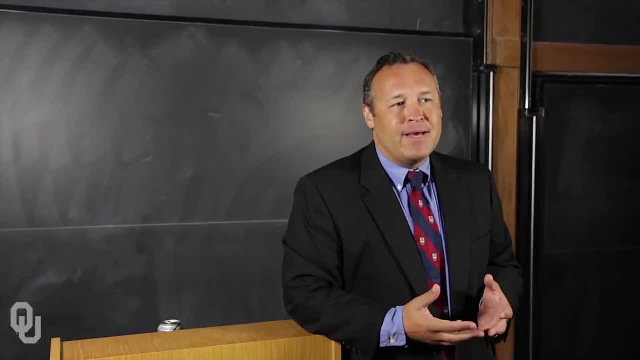 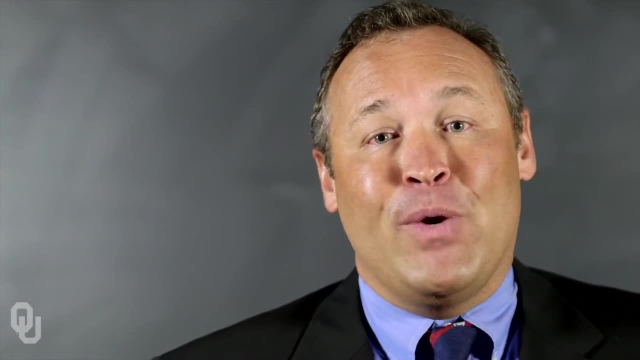 showing you how to calculate these statistics and help you understand how to get the numbers in the right place and how to get them all to add up together to get the right answer. Now, Mitch and I have been together for a long time. We actually met in graduate school. We studied together at